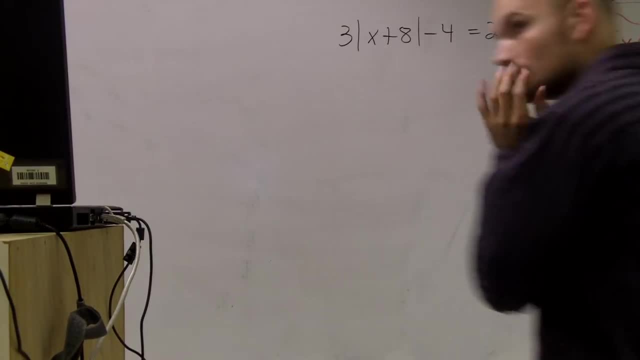 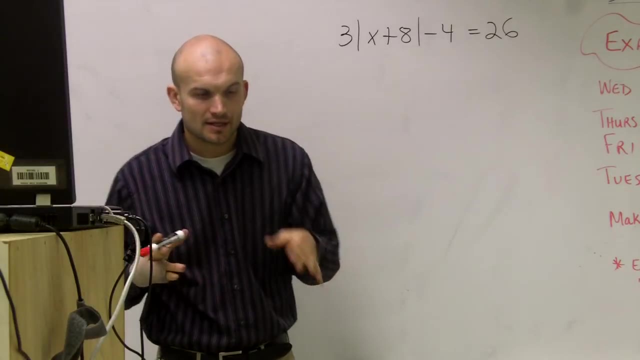 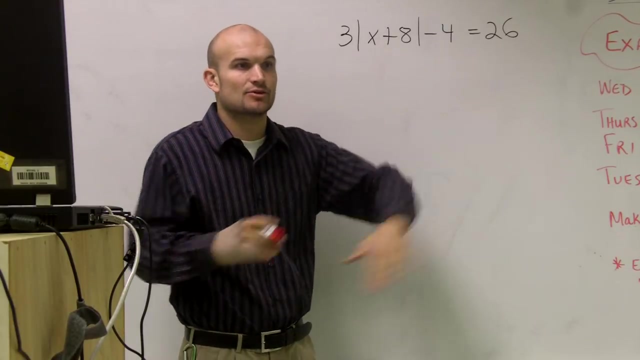 Okay, what I'd like to do is show you how to solve for this absolute value equation. Now a couple things you need to remember about absolute value equation. We need to leave our absolute value all the way at the end, So before we can do anything with the absolute 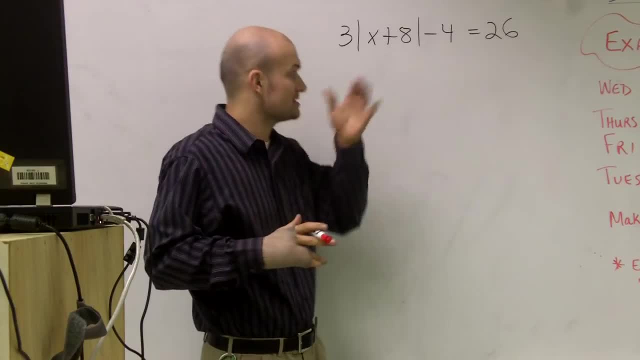 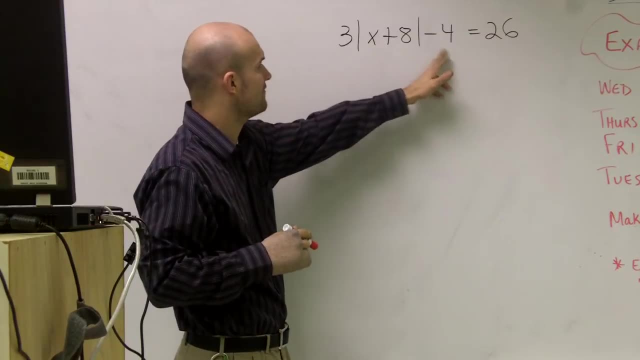 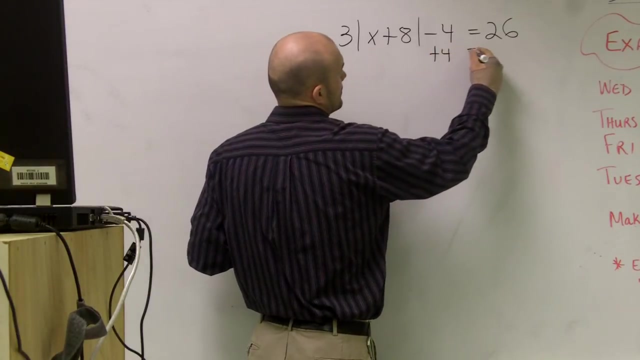 value equation. we need to isolate our function, which is the absolute value equation. So I need to get this by itself. So to do that, I need to get rid of that negative 4 and this multiplication of 3.. So to do that, I'm going to add 4 on both sides And then I'll have 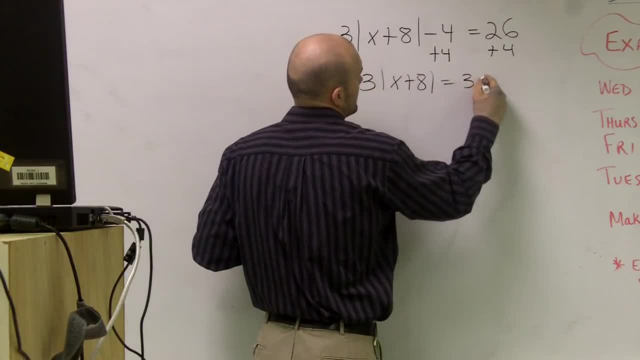 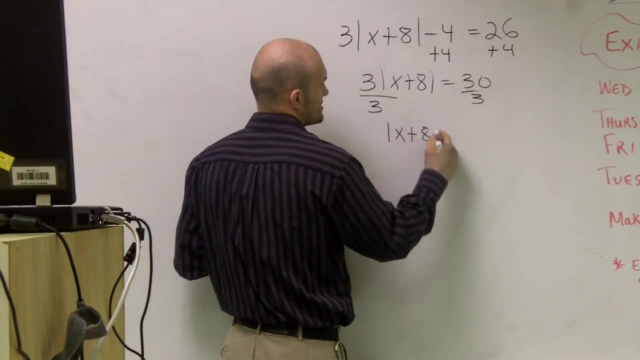 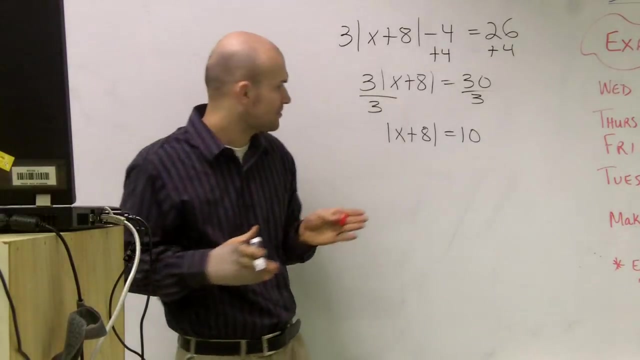 3 times x plus 8 equals 30. Then I'm going to divide by 3. And I'll have absolute value of x plus 8 equals 10.. Now that I have the absolute value of x plus 8 equals 10, I can now rate that into two. 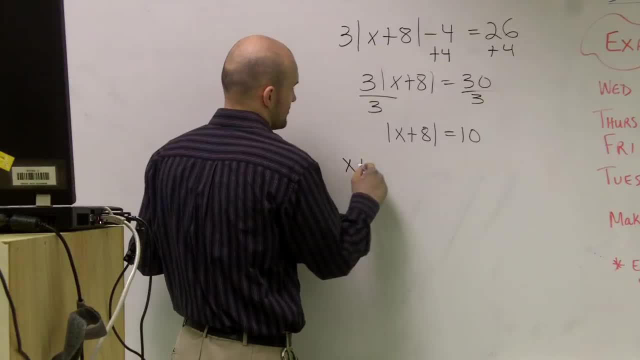 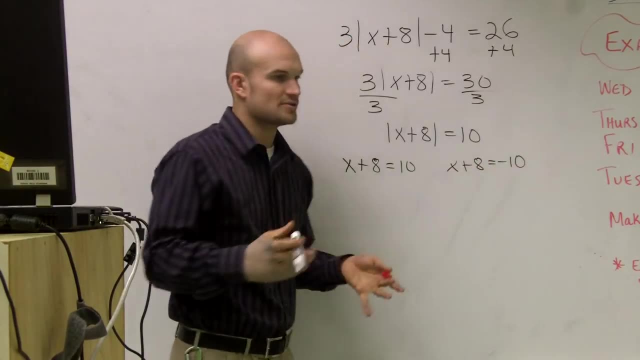 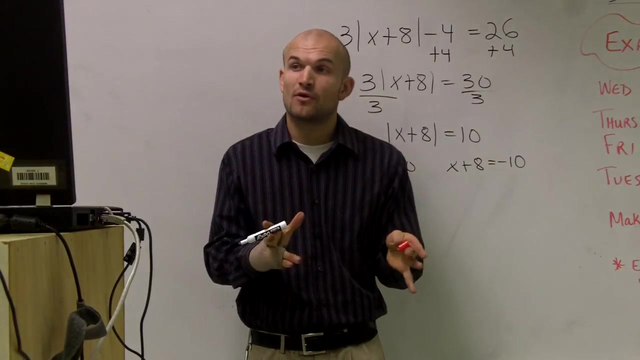 different equations. I can say x plus 8 equals 10 and x plus 8 equals negative 10.. Because remember an absolute value- the absolute value of negative 4 is 4.. And the absolute value of 4 is also 4.. So you need to make sure that you're taking this as a positive. 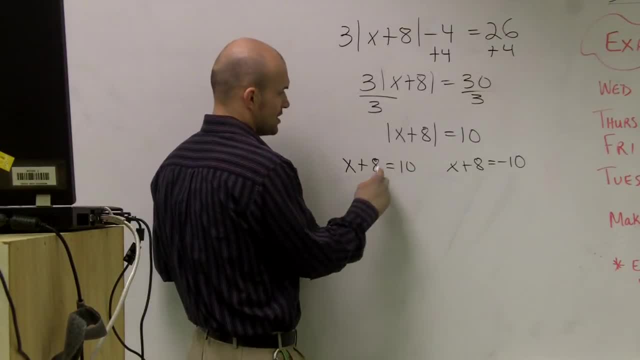 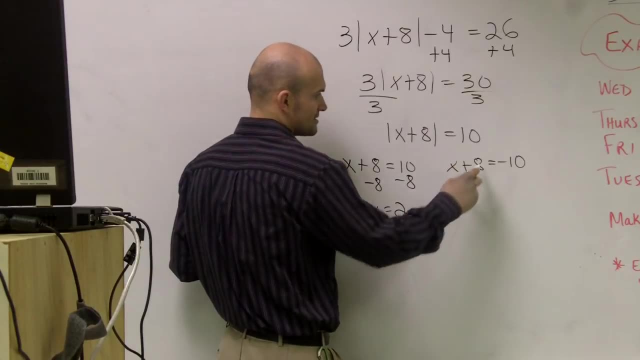 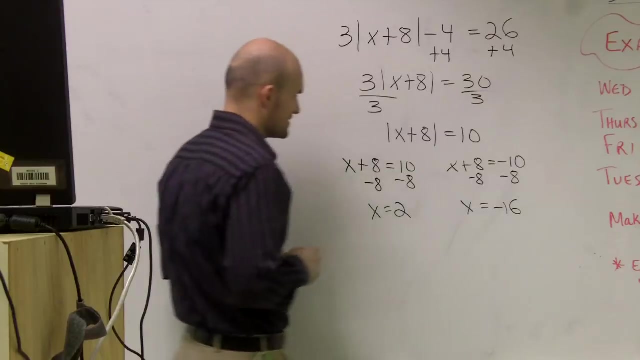 and a negative And solving it twice. So here to solve, for this one I'll subtract an 8. And therefore I get x equals 2.. And for this equation I'll subtract an 8. And I get x equals a negative. 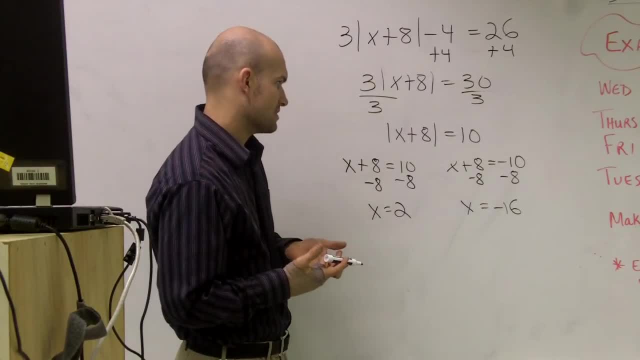 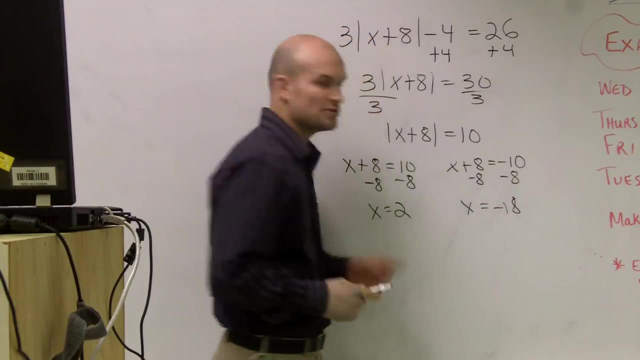 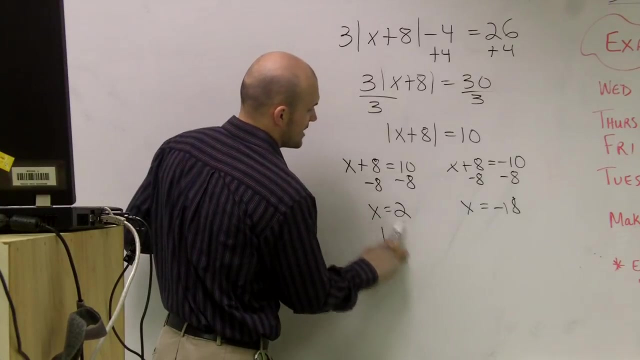 16. And we look at that, I'm sorry, Subtract 8.. Negative 18.. Not a 16. And now let's just go back and plug these back into our equation, Just to make sure they work. So we have x, I'm sorry, x is now equal to 2.. So 2 plus. 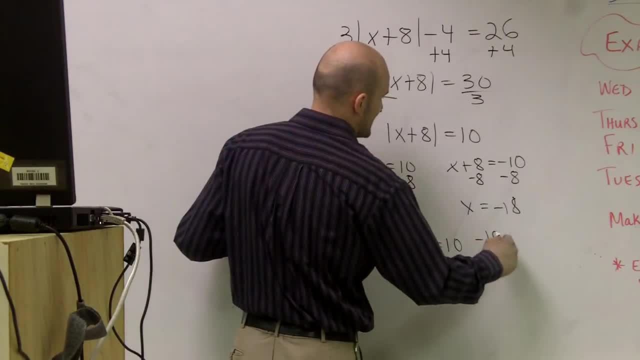 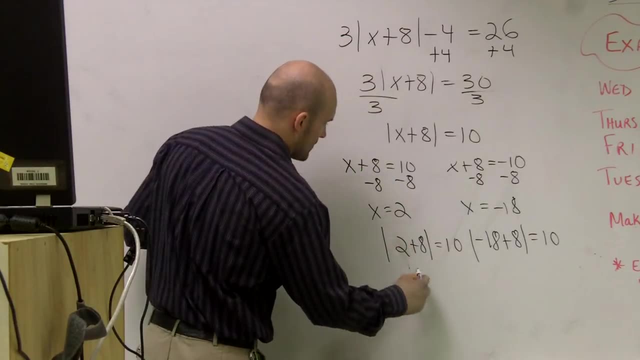 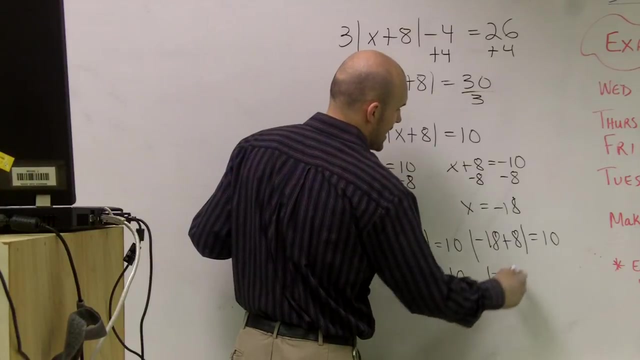 8 equals 10.. And negative: 18 plus 8 equals 10.. Well, 2 plus 8 is 10.. Absolute value of 10, we know obviously is 10.. And then negative: 18 plus 8 is a negative 10. Absolute value.